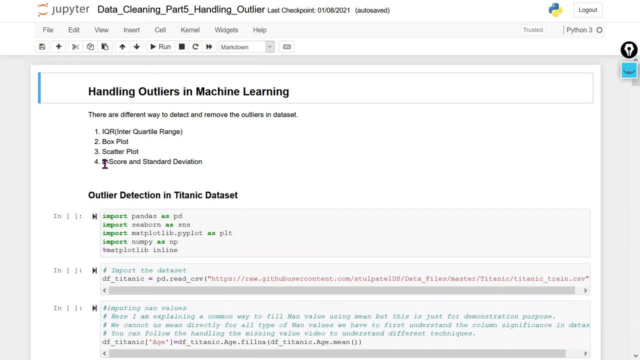 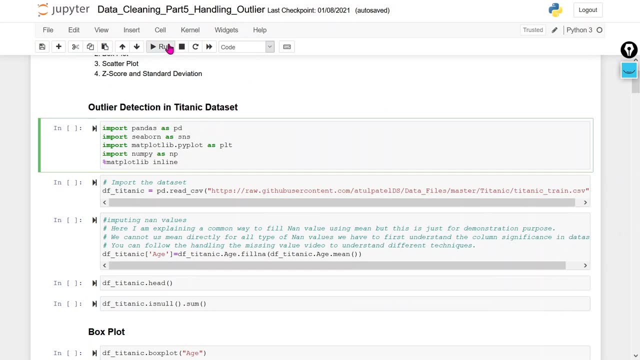 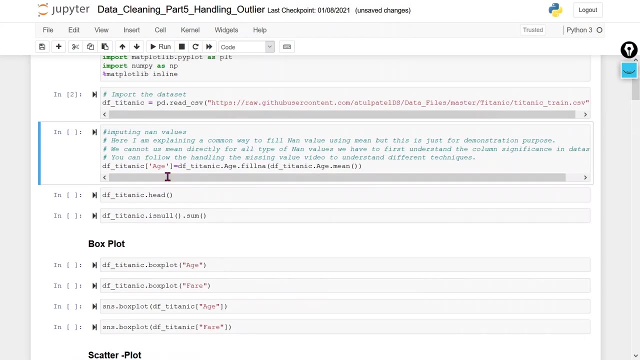 and at last we will discuss z-score and standard deviation. So, first, I am going to import the required libraries, I am going to import the titanic dataset here Now, as we have the null value in our dataset. so what I am going to do, I am going to 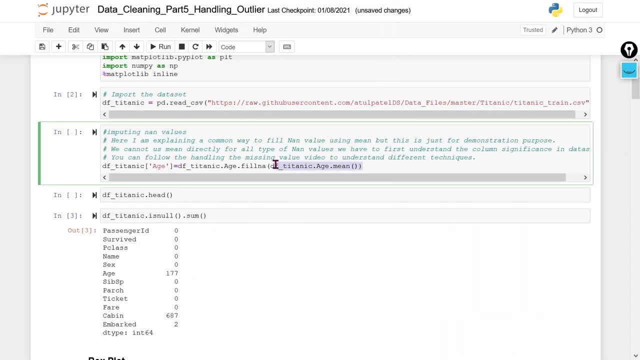 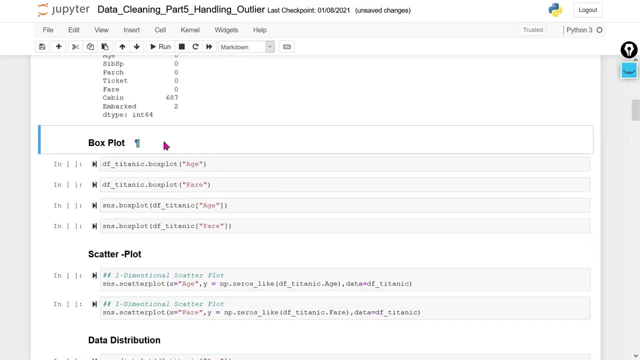 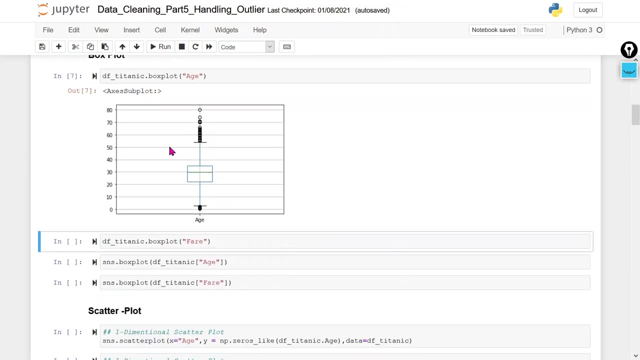 impure this null value with the help of mean of the age column. So you can see this value has been replaced. Now I am going to use the box plot to check the outliers. Now you can see these black dots are the outliers. We will discuss box plot in details later on. 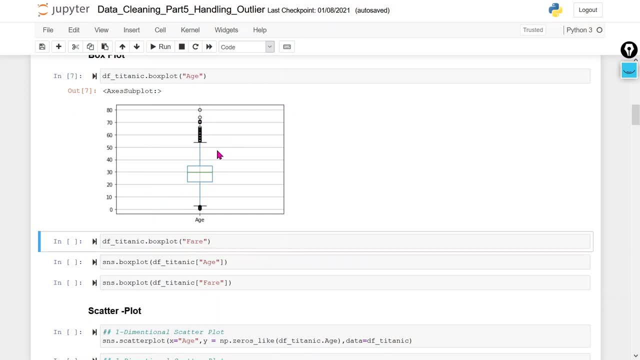 but you can see how you can visualize the box plot and how you can like see whether we have outliers in our dataset or not. So let's see how we can visualize the box plot and how you can like see whether we have a outliers in our dataset or not. 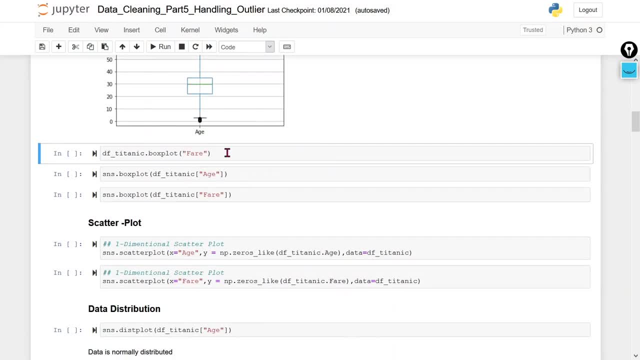 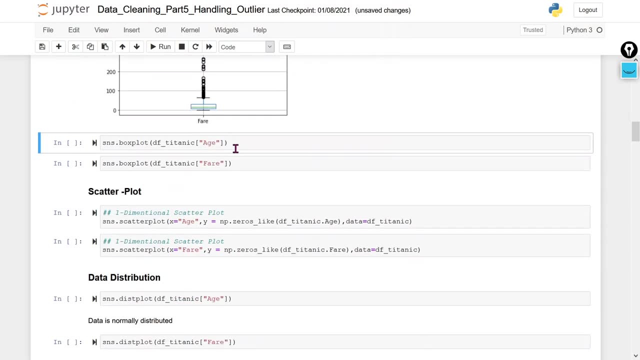 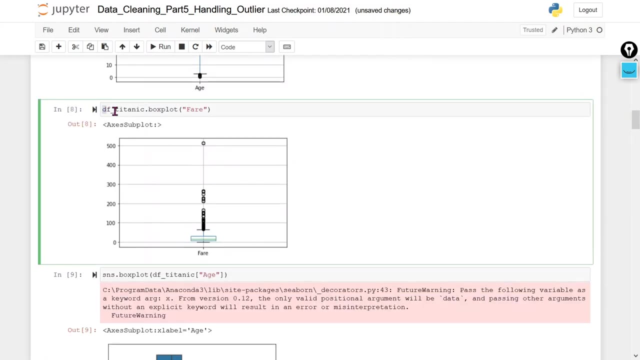 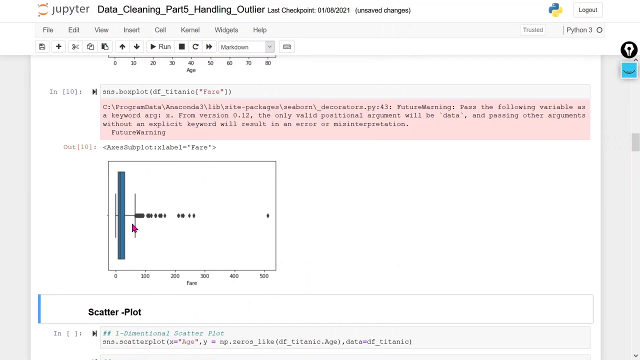 by using the box plot. Same thing we can use for the fair. You can see. these are the outliers. Now we can use the different method to plot this. Here I am using the data frame. Now I am using the c1 library. So for the fair, we can see. these are the outliers. Now I am using the scatter plot. 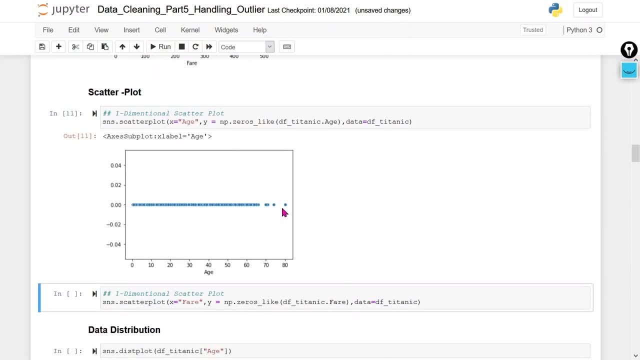 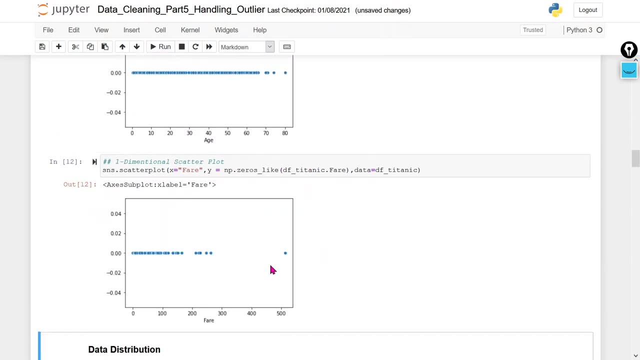 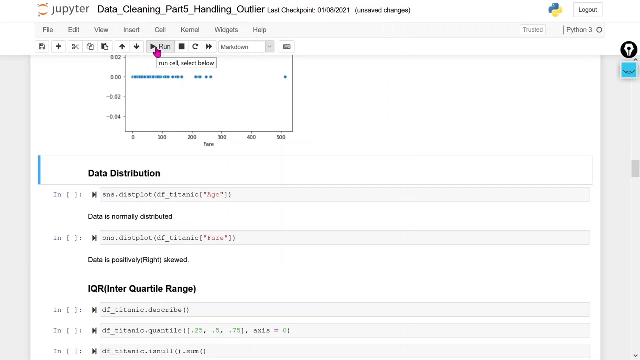 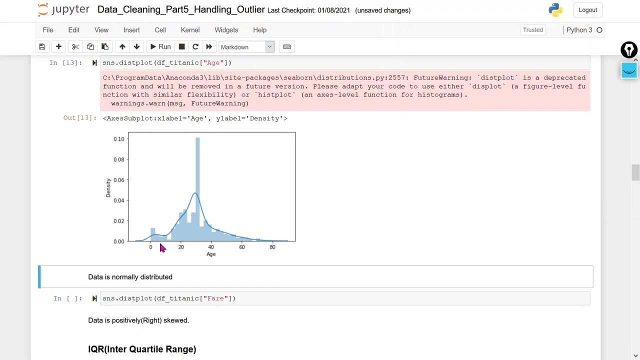 Now I am using the scatter plot. You can see in the scatter plot these values seems like the outliers and for the fair value we can say this value will be treated as a outliers. Now I am going to visualize the data distribution for both columns, age and fair. So here we can see age column data seems like the normally distributed. You can see, But fair is not the best option. 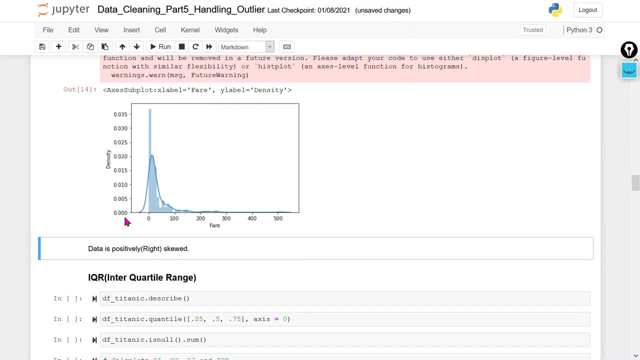 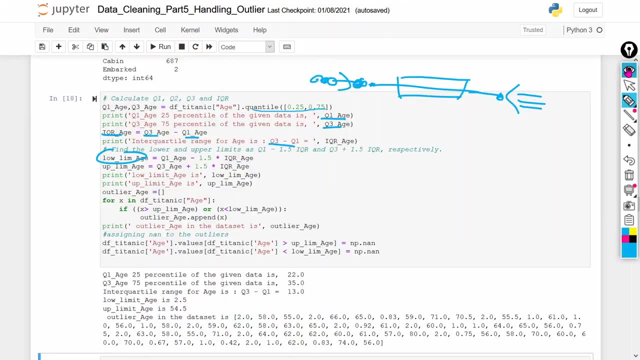 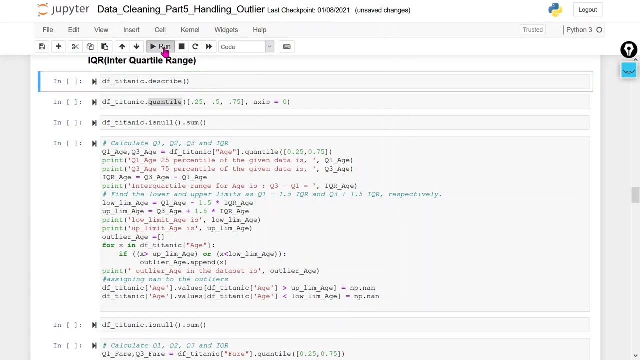 see, but fair column data. this is not the normally distributed. it is seems like positively skewed or the right skewed data. so now i am going to use the interquartile gains to calculate the outlier. so first i am going to describe the titanic data set. it means all the statistics of this data set. 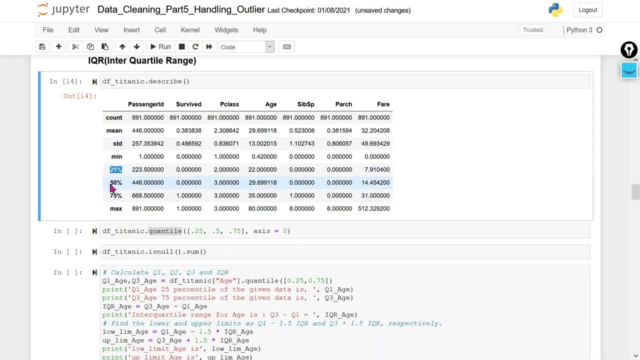 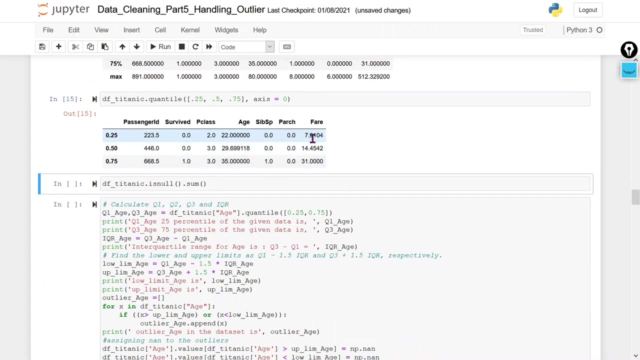 you can see we are getting 25th, 50th and 75th percentile of all these data. it means if we want to check what is the 25th percentile, that would be 22 for the h column. if we want to calculate only for the numeric data, we can use that. you can see. we can get the statistics for the numeric data or. 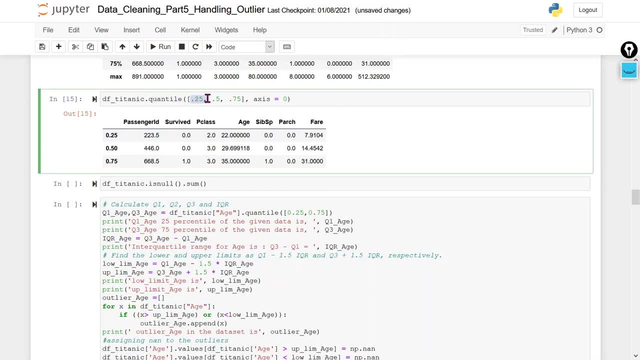 we can use the quantile to check the 25th, 50th and 75th percentile directly by using the quantile method. so these things we use to calculate the iqr. so let's check what is the iqr first, that this is your, our data set and we created. 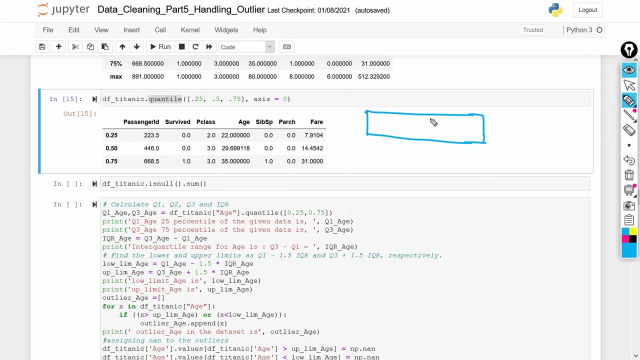 a box plot by using that particular data. so this is your median and this is your q1. this is your q3 and median it mean this is your q2 and then after that, this is your minimum value. this is your maximum value. so this is your lower limit and this is your upper limit. it means whatever the value we have. 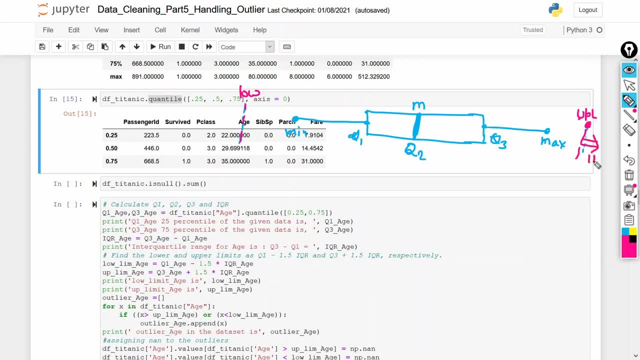 after this value upper limit, those value will be treated as a outlier. and whatever the value we have after this lower limit in the left side, Those value will be treated as a outliers. It means this value, from this to this, will be your Q1 minus 1.5 IQR, and from this to this, this will be your Q3 plus 1.5 IQR. 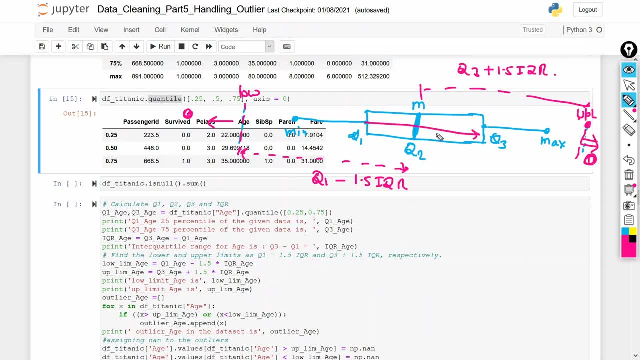 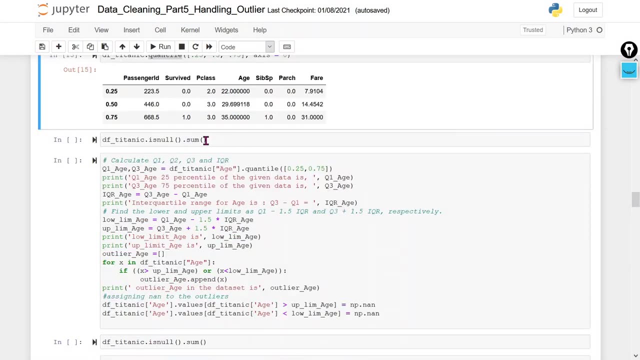 Now how we calculate the IQR. IQR is this: It means Q3 minus Q1. So this range is called as a interquartile range. So by using this particular things, we calculate the outliers. So here what? 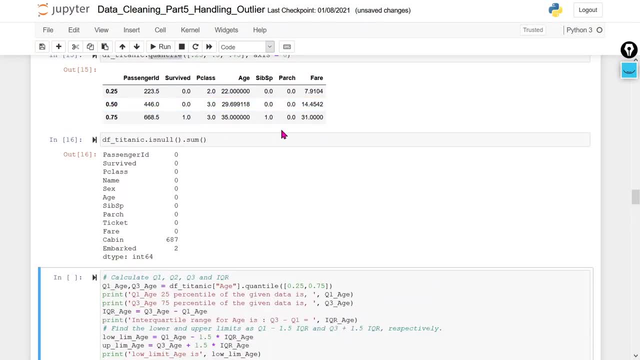 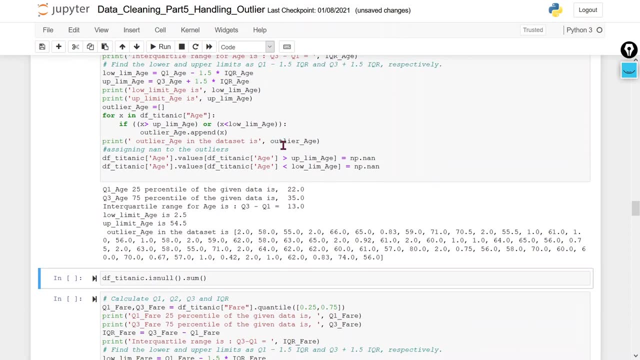 I am going to do: I am going to check whether we have any null value or not. We don't have any null value, So I am going to run this particular complete code. So what I am doing here: first I am going to check the outliers. So I am going to check the outliers, So I am going to check. 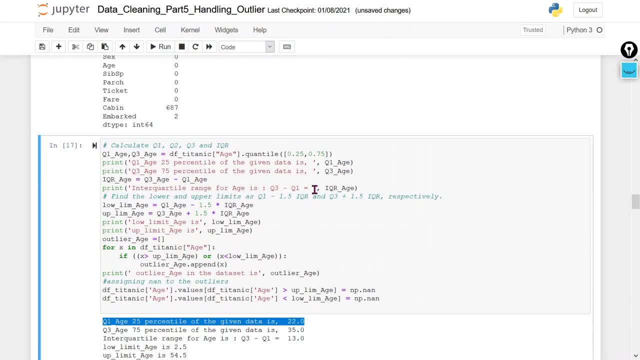 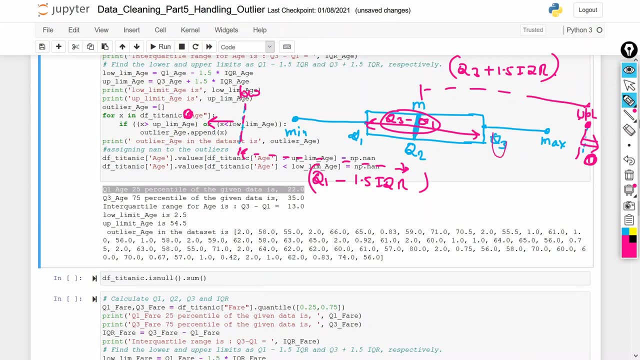 the what is the Q1. It means your, this particular Q1.. Then Q3, it means this particular Q3.. Then interquartile range: Q3 minus Q1,. this Then lower limit: it means this particular limit: 1.5 Q1. 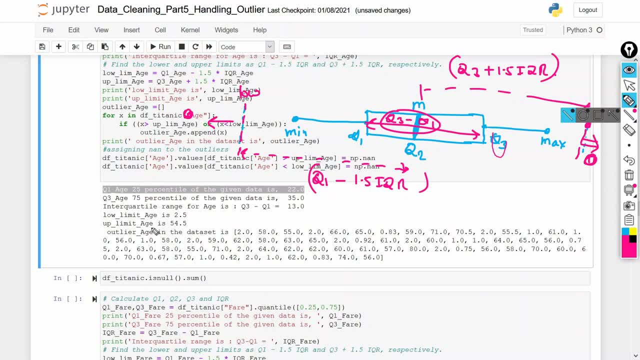 minus 1.5 IQR and upper limit Q3 plus 1.5 IQR. So why doing this? We are able to get all those details. Then how we calculate the outliers, All the value after this and all the value after this. So, whatever the value we will get in this particular 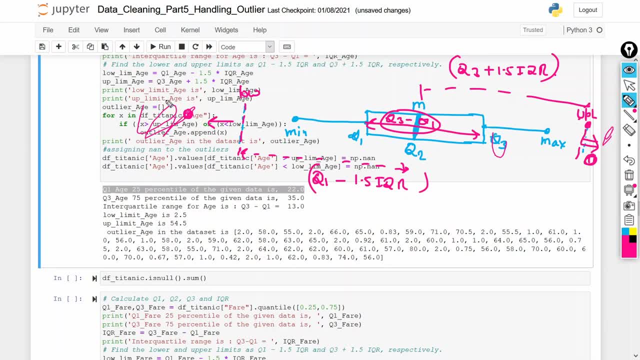 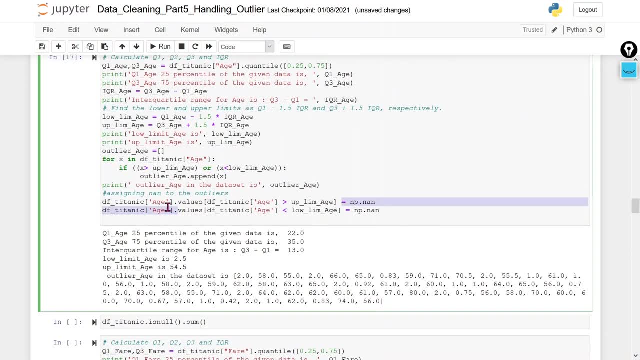 range, this range and this range, So those value will comes under the outliers Same thing. I am getting here Now what I am going to check, Because here, whatever the outliers value we will get, we are going to replace those outlier values with the NAND value. 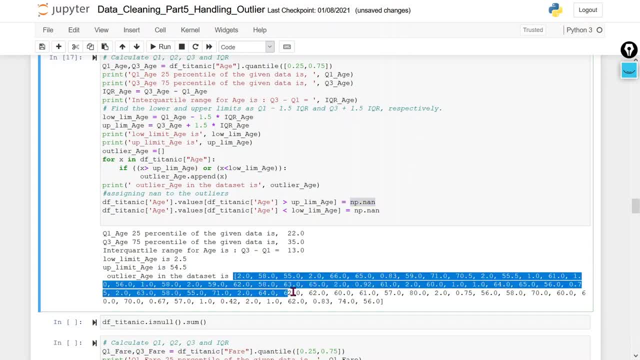 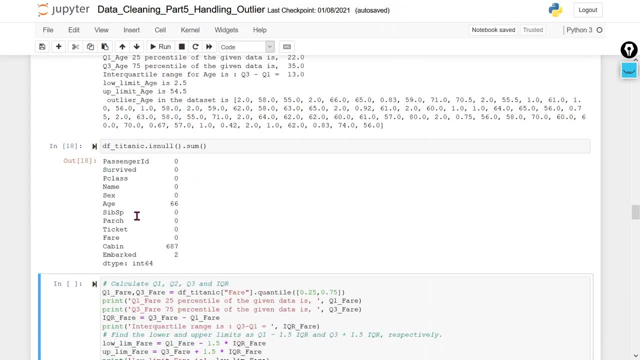 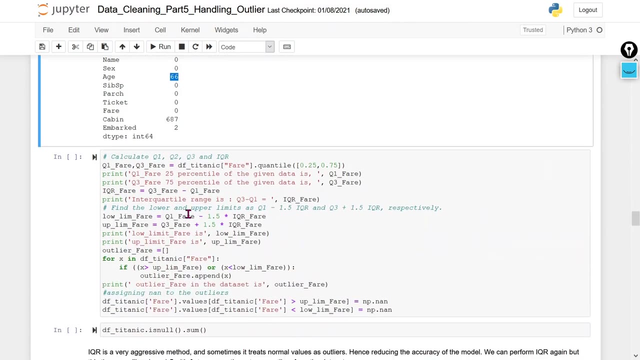 It means if we have like 10 these values, we are getting these values. So we are replacing these values with NAND value. That's why I am going to check the null value So we can say that there are 66 outliers. Those values have been replaced with null value. Now we are going to 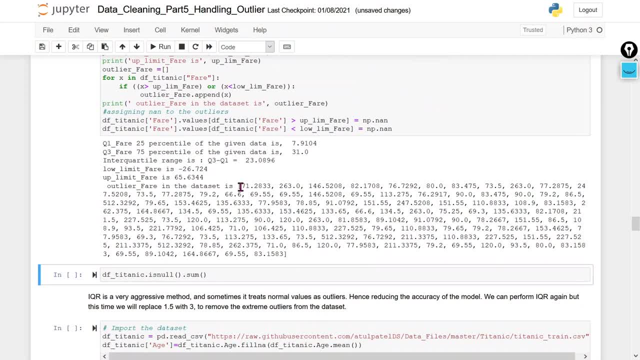 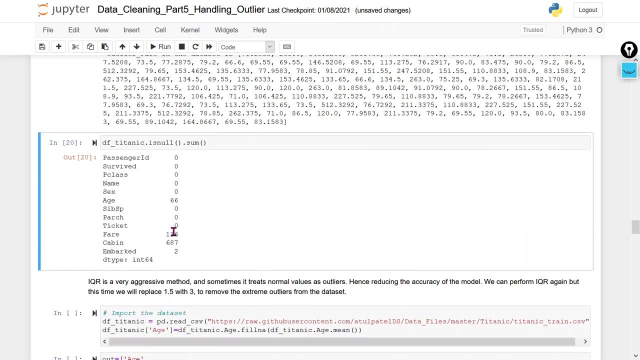 check the outlier in the fair column: Same thing. So here I am getting the outliers. So again I am going to check the null value. Yes, we have 116 outliers In the fair column and those value have been replaced with null value. As we know, IQR is a 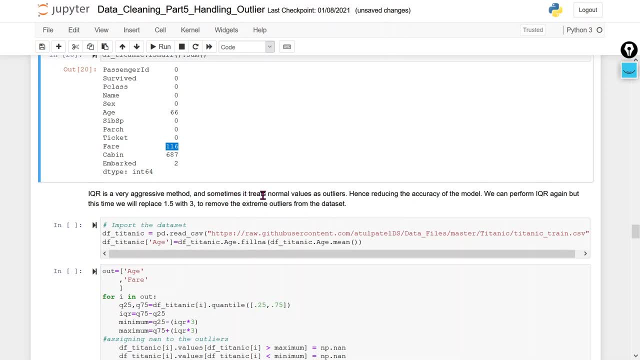 very aggressive method and sometime it treats normal value as outliers Because we are using the 1.5. that is very low range. So that's why we try to use different, different value at 1.5, 2,, 2.5, 3.. So this way we can remove some extreme outliers from the data set Might be. currently we 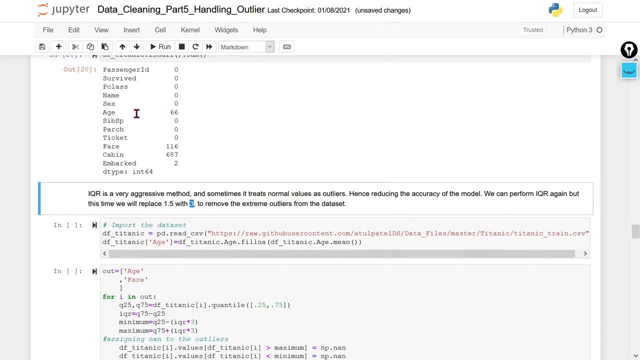 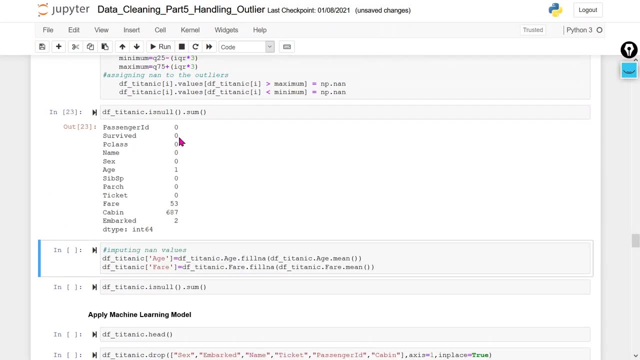 have 26.. If we will use 3, might be we can get some less value. Let's check it Now. I am going to use the 3.. Now you can see we are getting only 53 and here only one value. So I am going. 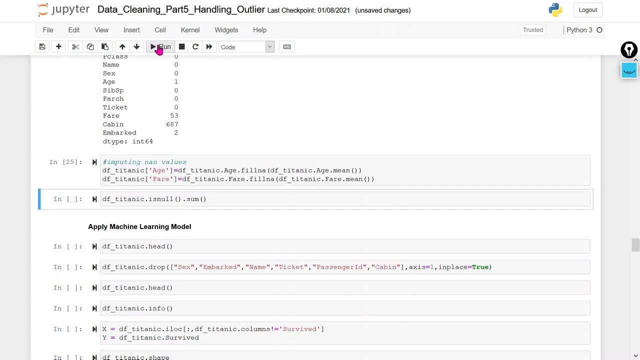 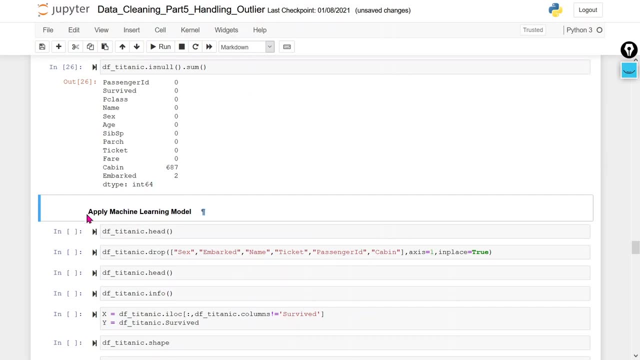 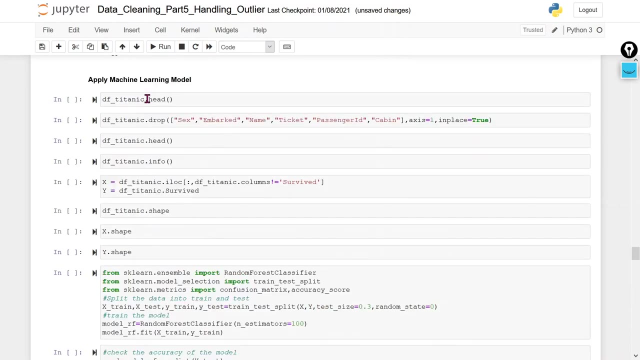 to replace these NAND value with the mean value. Now I am going to check the null. We don't have any null value. So what I am going to do, I am going to apply one machine learning model on this integrated data set. It means where we have removed the outliers, So I am going to just 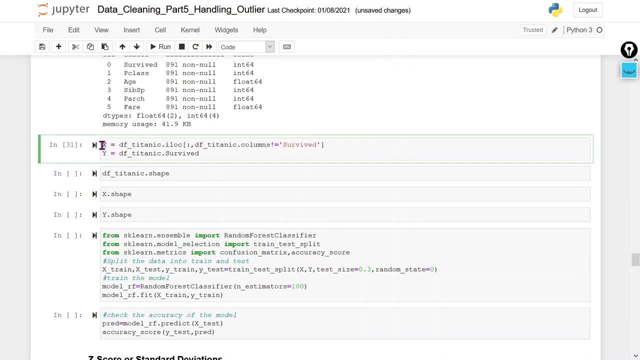 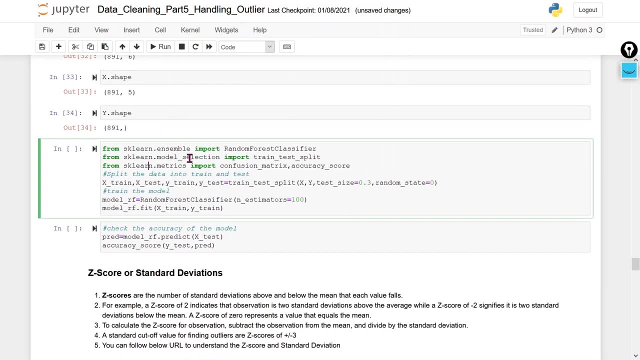 check. Now you can see I am dividing the x and y. This is your feature, this is your levels. Now, again, I am going to check the shape: X is this, y is this? So here I am going to use the random. 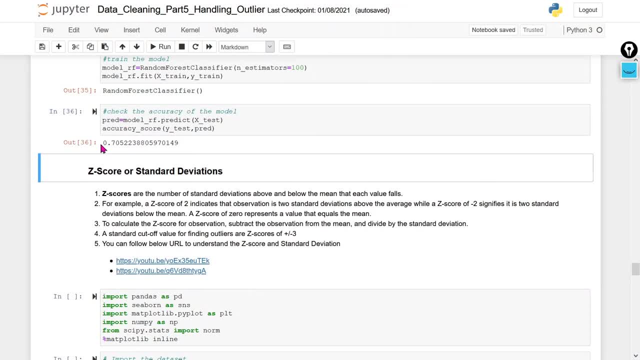 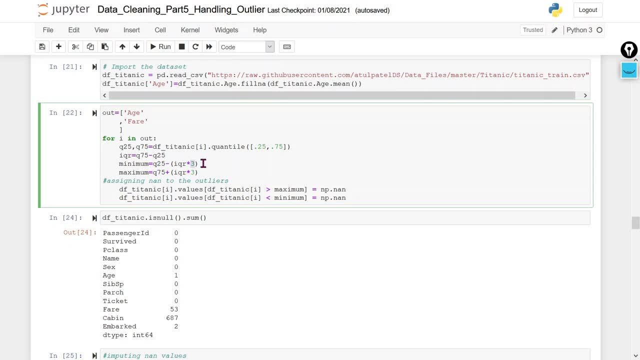 forest classifier. So you can see what I am getting: the 70% accuracy currently When we detect the outlier with the help of IQR, multiplied by 3.. If I use 1.5, you can see 1.5. in that case, let's check what would be the accuracy we will get. 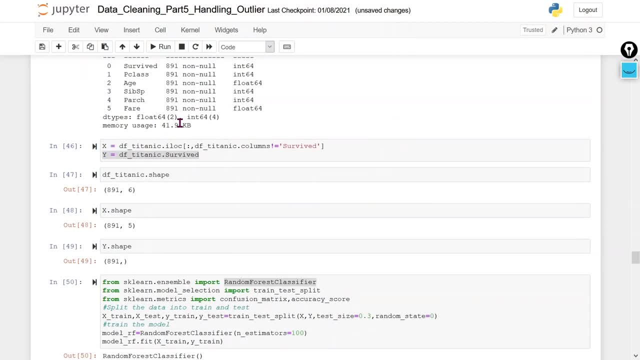 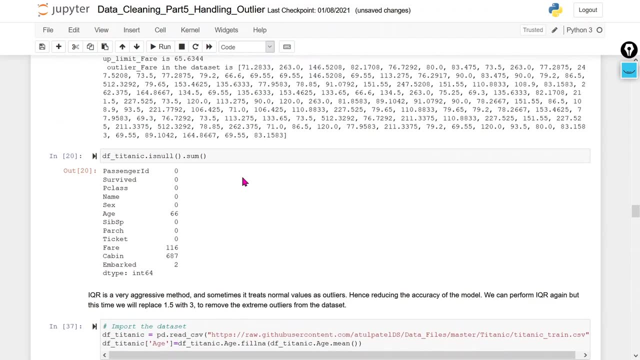 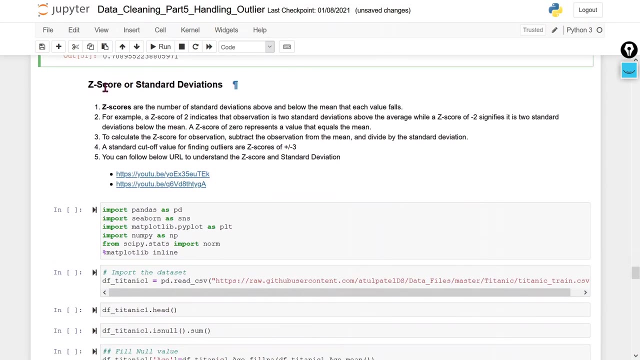 just we are getting almost the same accuracy, so this is not causing any too much issue. but if we have some different data set, we can try these things, just changing all those things. now, what I am going to do, I am going to use the z-score, or standard deviation, to 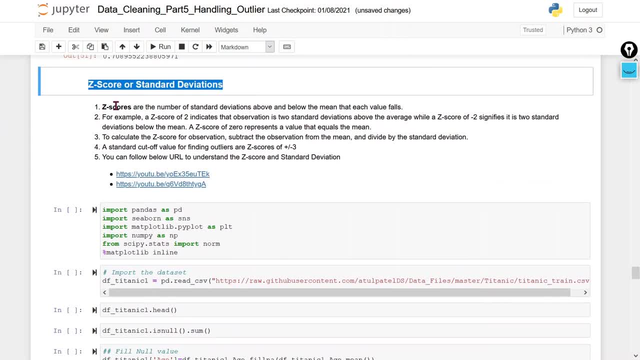 detect the outliers. so what is the z-score? z-score is the number of the standard deviation above and below the mean that each value fall. it means, if our data set is normally distributed, in that case, let, this is our data, okay, and this is your. our mean and mean is equal to 0 and standard deviation is equal to 1. 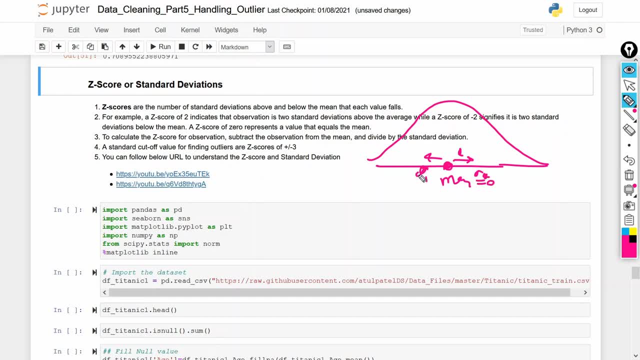 this is your sigma 1. sigma 1, first standard deviation. this is your first standard deviation, so this will be called as a. z is equal to 1. z-score is equal to 1 for the standard normal distribution data set. if you want to understand what is the z-score standard deviation I have 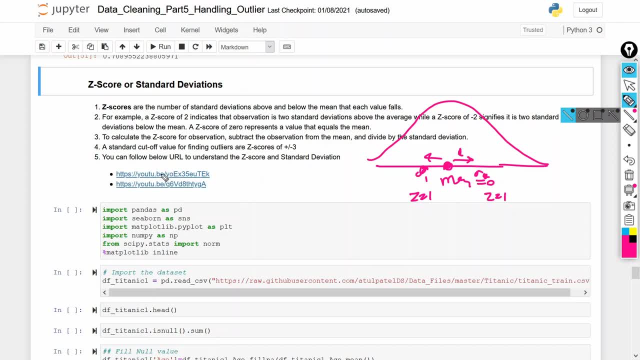 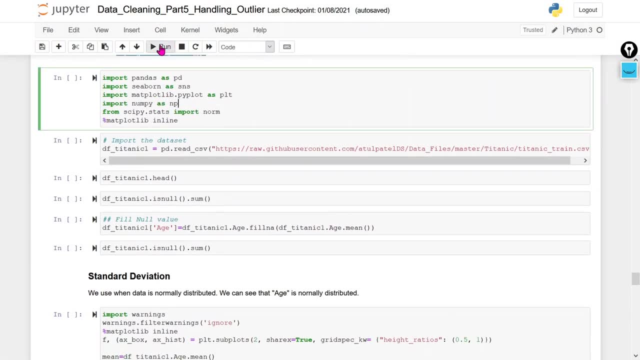 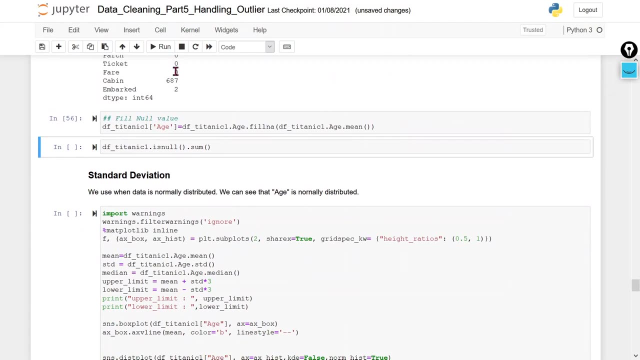 mentioned the youtube video link which I have created. you can follow this link to understand what is the z-score, what is the standard deviation. so now I am going to import these required libraries. first, this is your data set. here I am going to impute the missing value now. 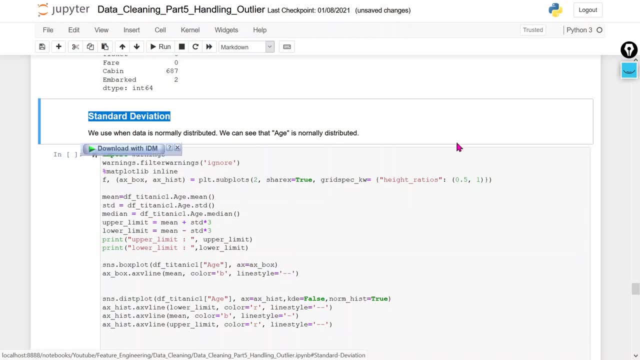 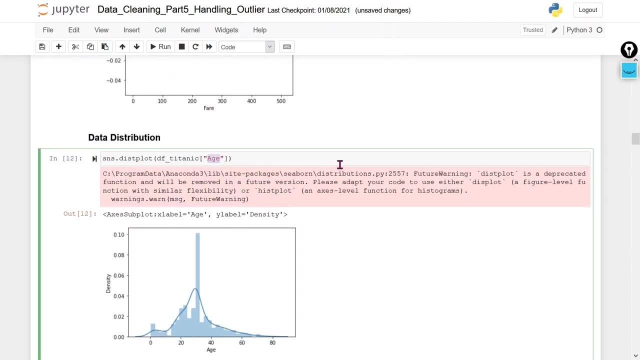 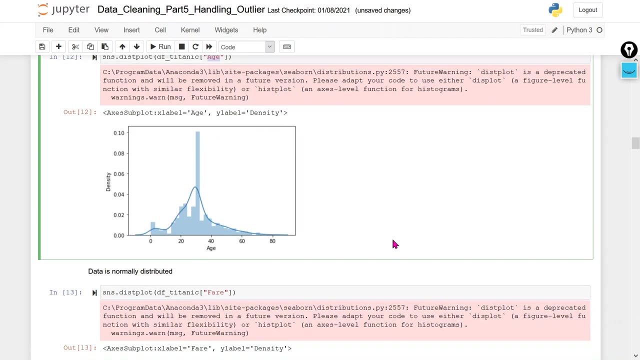 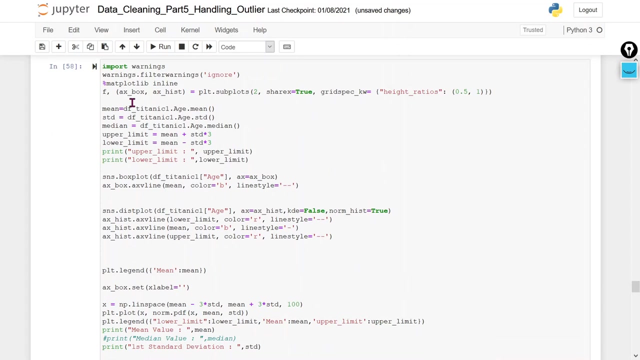 what I am going to do. I am going to use the first standard deviation. so, as we have seen here, h column- h column data set is normally distributed, so we can use the standard deviation or z-score for this data set. let's check how we can use that. so I am going to run this complete code. I am not going to explain all. 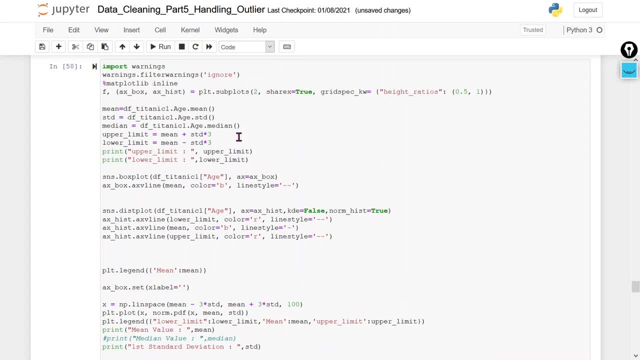 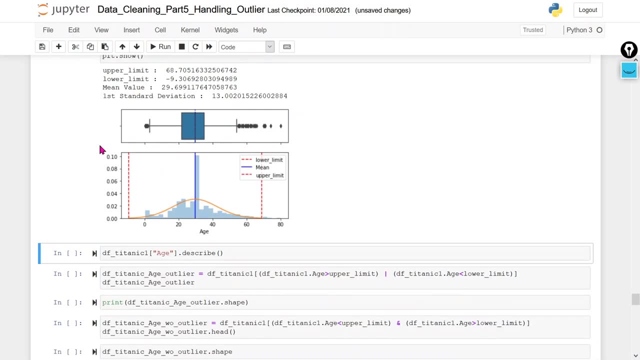 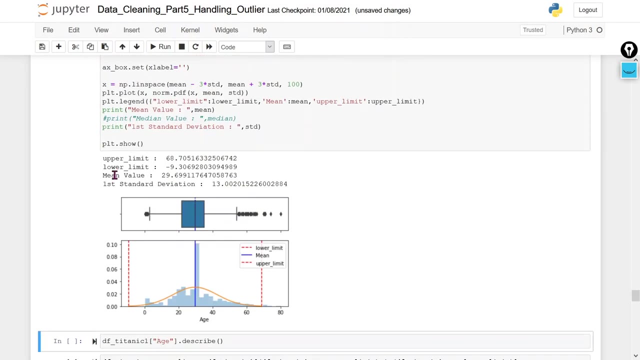 these code because if I will explain then this video will be too long. so if you want, I will explain in a separate video. so here what I am going to do. I am going to explain how the standard deviation calculate the outliers you can see here. first we are going to check the upper limit. this is your upper limit, this is your lower. 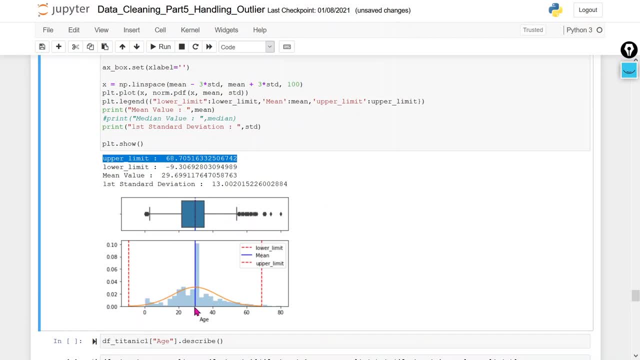 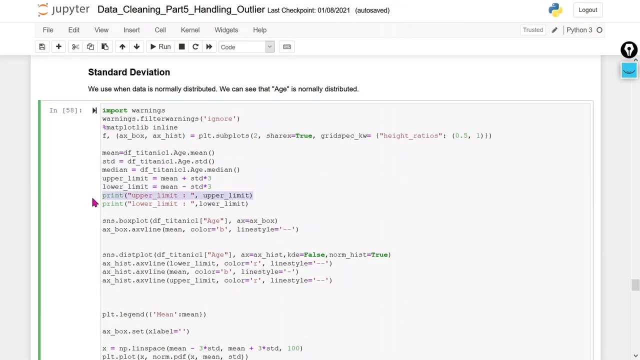 limit in the standard deviation. this is your mean. so first I am calculate the. what is the mean value? this is your mean value, 29.. this and what would be the upper limit? let's check it. upper limit is this. so what is the upper limit? upper limit is mean plus. third standard: 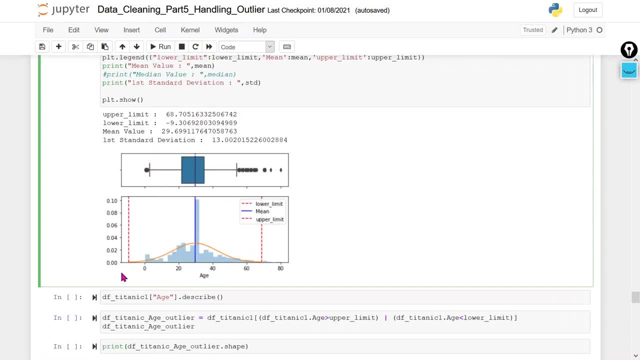 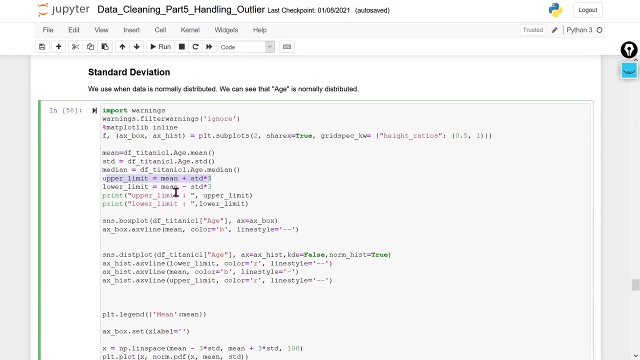 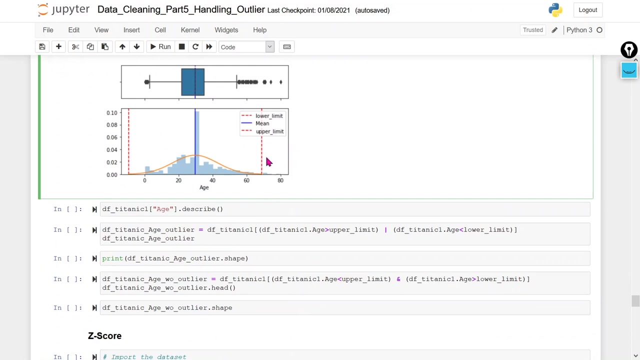 deviation. so this will be your upper limit. it will mean value. what would be the mean value? we will calculate that. how we will calculate the upper limit? this three standard deviation mean plus three standard deviation mean minus three standard deviation for the lower limit. this way we will calculate the upper and lower limit. so whatever the value we will get after. 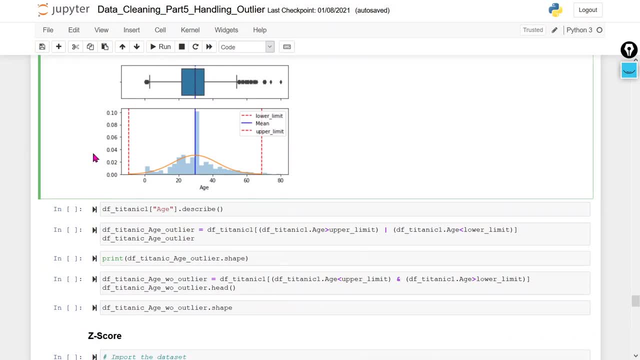 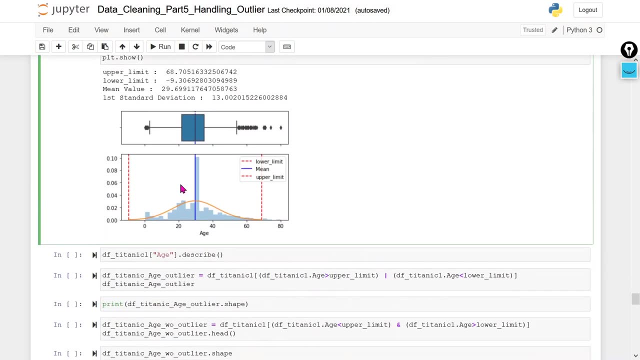 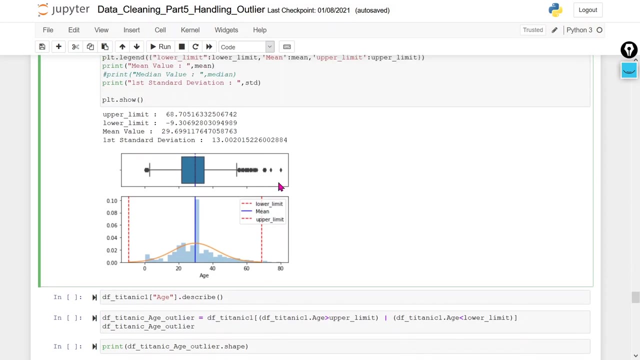 this. it means right side after this upper limit and left side of this lower limit, those value will be treated as your outliers. then after that, this is your median. median mean will be equal here. if you see, here there are very less value we are getting as a outlier. 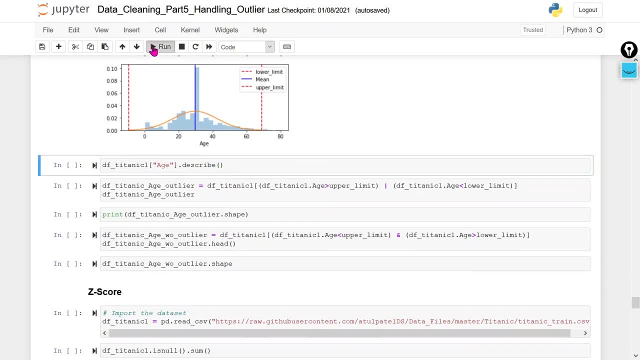 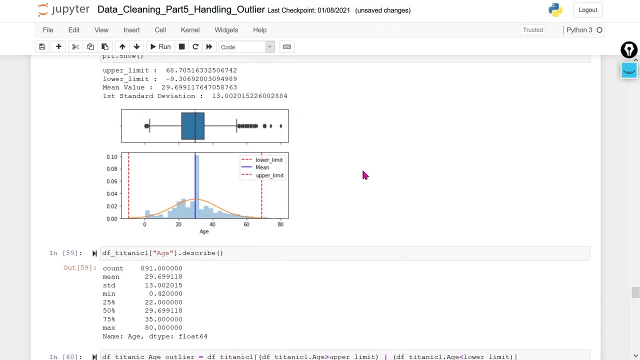 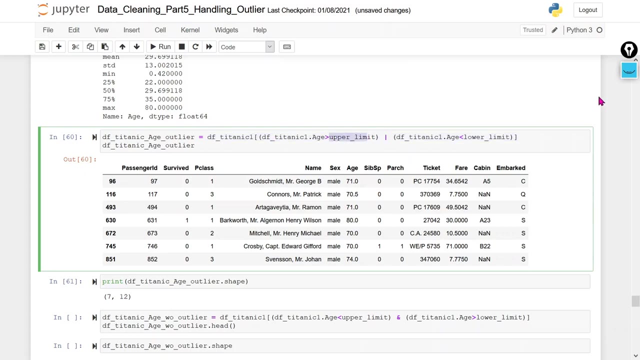 in each column. so let's check how many values we get. you can see there are only seven values we are getting. we are getting only seven values. what I am doing, I am using the OR condition here. it means right side and left side data. I am combining both side data here, so we are getting. 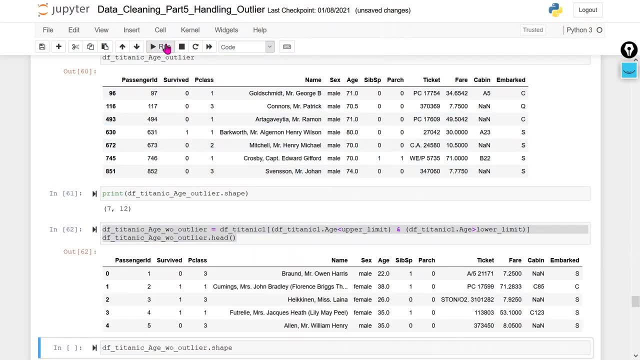 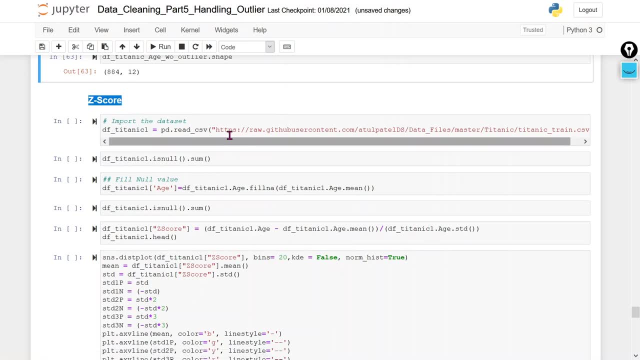 seven outliers and what are the remaining value we have? you can see that 884.. now I am using the Z score. Z score we apply on the standard normal distribution data set. so first we have to convert our data set into a standard normal distribution, standard normal. 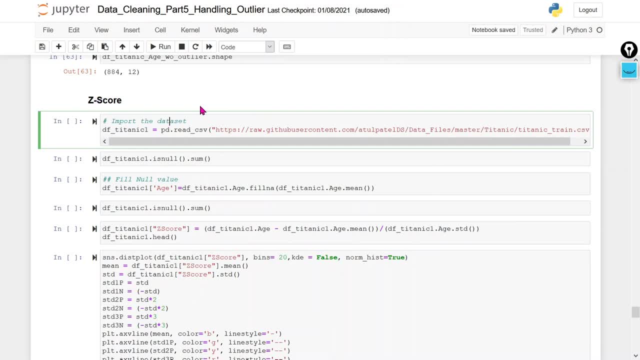 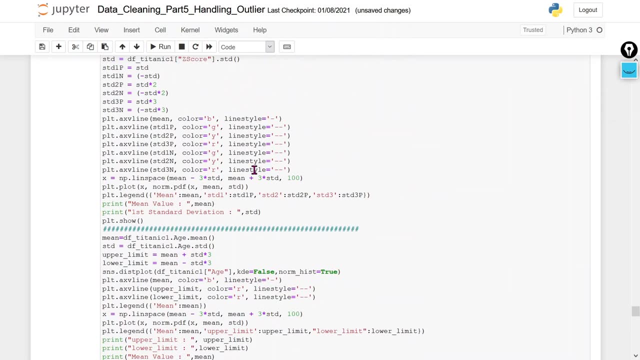 distribution. data set means where mean is equal to zero and standard deviation is equal to one. so let's do it first. here you can see that what I am going to do, I am going to convert our data set into a standard, normal distribution. how we can do that, there is a very simple. 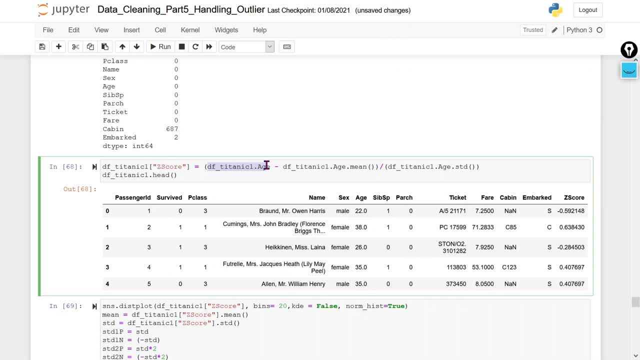 formula for that Z score. this is your x minus mu. mu means your mean value divided by sigma. so we are calculating the Z score for each rows, this particular Z score, and we will use this z score as a h column, because we are going to use this z score for our h columns. 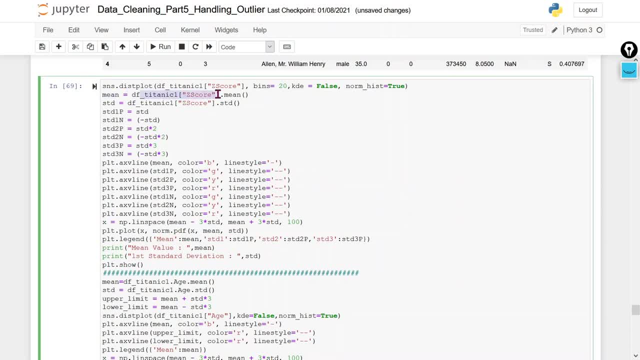 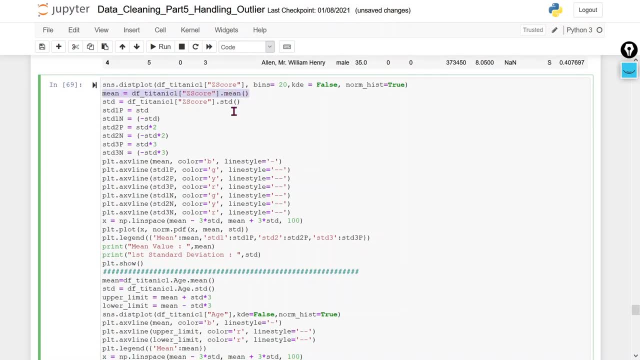 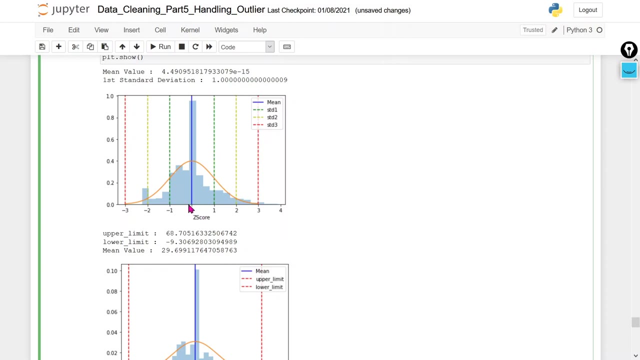 see that mean is equal to df titanic one z squared. it means this is your h column minus mean. so mean of the h column after computing the z score. so you can see here this is your mean. in the standard normal distribution data set we have, mean is equal to zero and all the value. 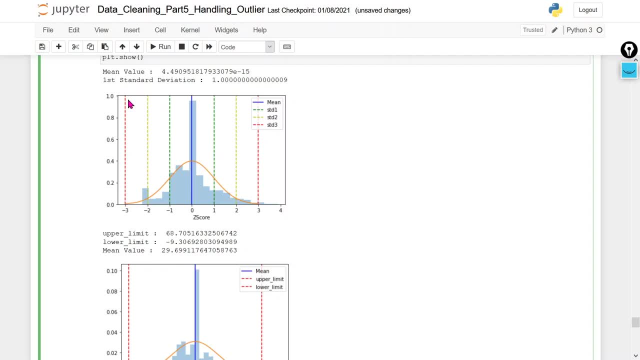 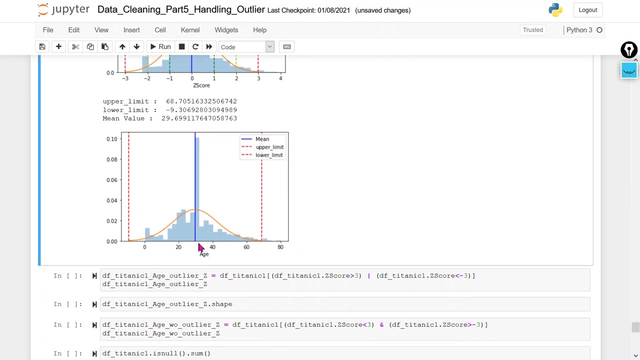 after third standard deviation will be treated as a outlier. It means this is your third standard deviation, All the value left this side and all the value right this side, This side and this side, Those value will be treated as a outliers. So here same thing. This is your 29.. This is: 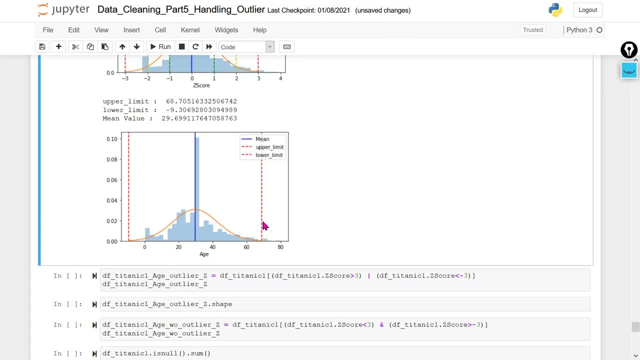 your mean value 29.. It means all the value from this value, all the value right side from this value. Those value will be treated as your outlier And all the value left side from this value will be treated as your. all the value left side from this value will be treated as your. 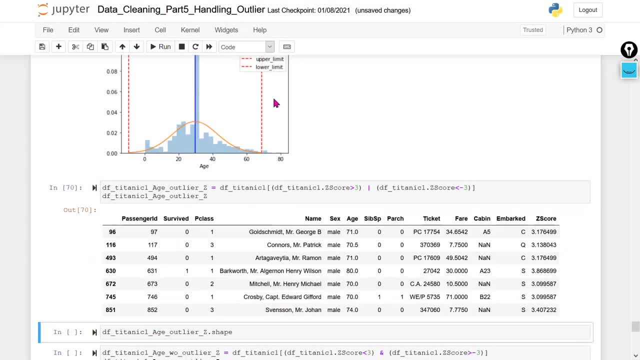 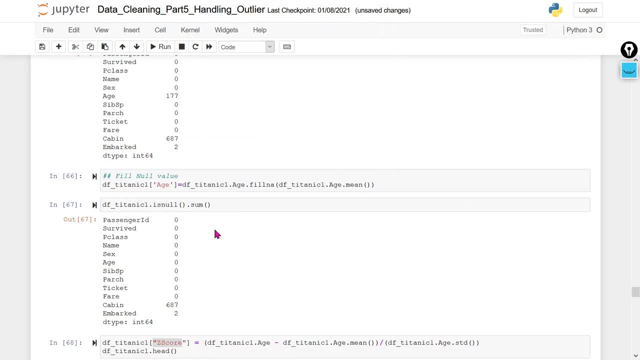 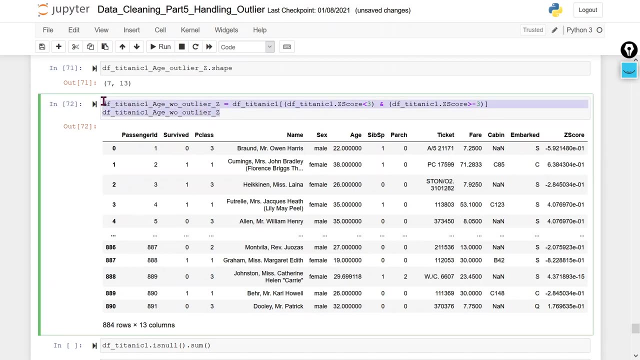 outliers. Now I am going to check what is the shape of the outliers. You can see that we are getting 7 outliers, Same value as we are getting with the standard deviation. Same thing we are getting with the z-score. Now I am going to check how many remain data. 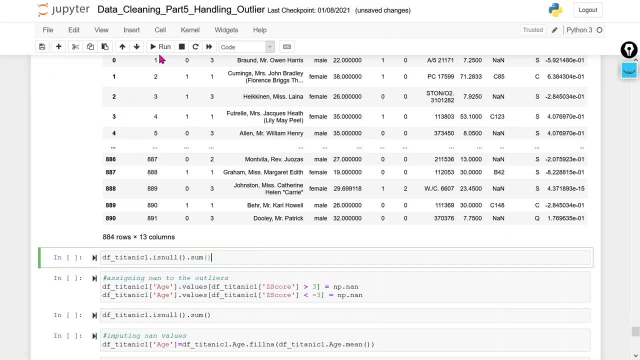 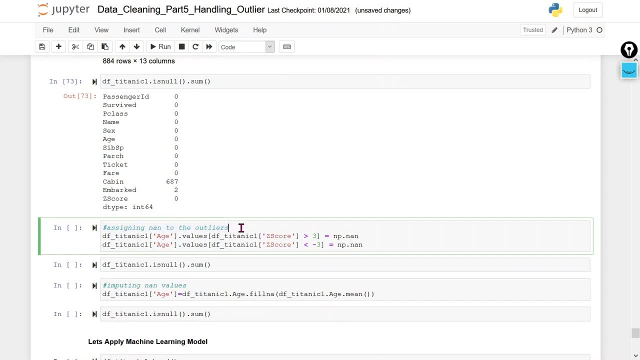 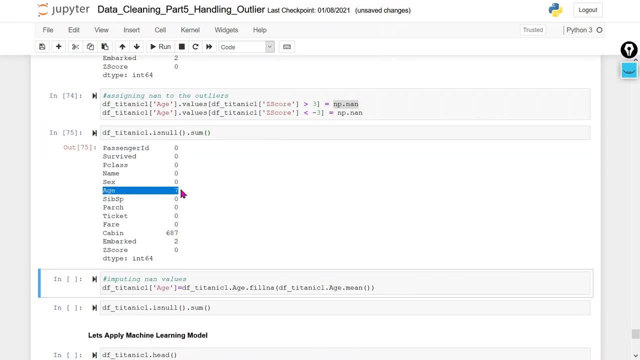 set we have. We are getting 884.. Now I am going to check the null value. We are not getting any null value. So what I am going to do, I am going to check the outliers and replacing those outlier values with the null value. After that, I am going to check the outliers. We have 7 outliers. 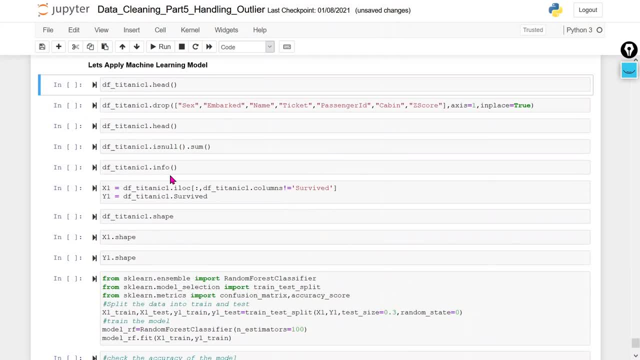 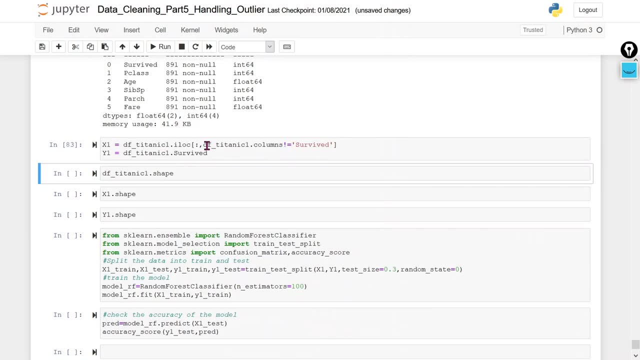 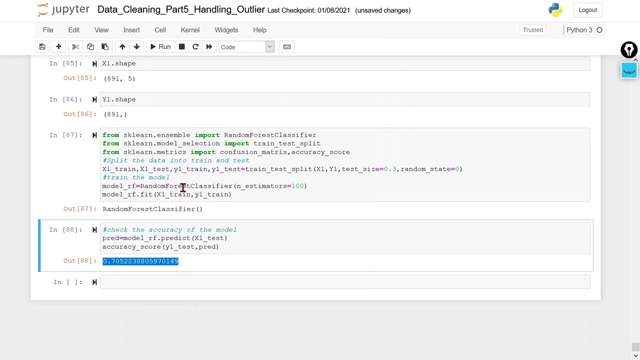 I am replacing these values with the mean of the h column. Now I am going to apply the machine learning model here, Same thing which we have already applied in our previous steps. Now we can see that we are getting the around 70 percent accuracy. It means by using the IQR and 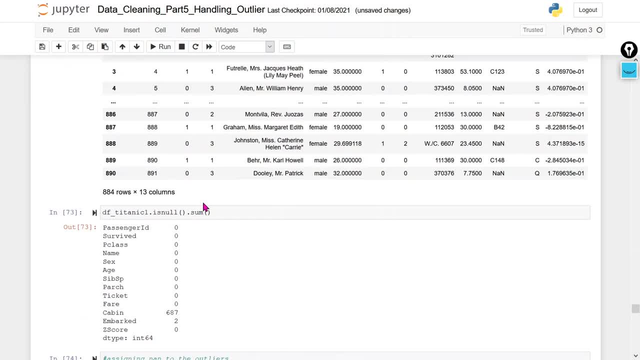 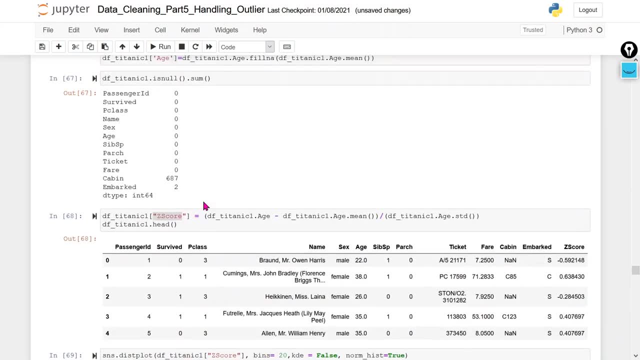 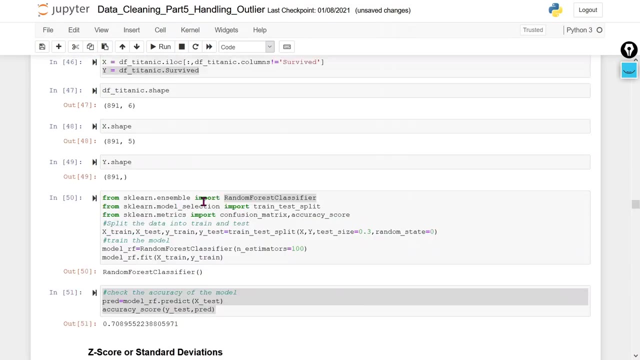 by using the standard deviation we are getting the same accuracy, But it depends on the data set. If you have some different data set might be you can get some different accuracy. So this way we can use z-score interquartile range, standard deviation box plot, scatter plot to calculate. 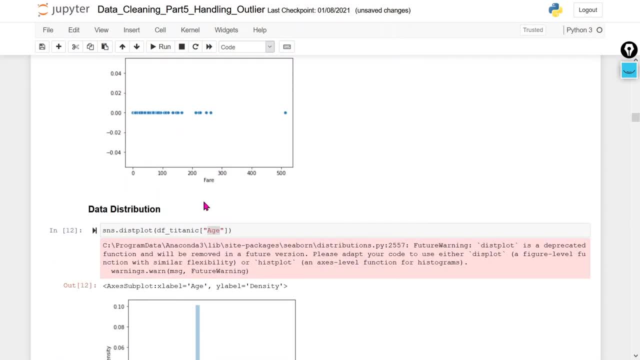 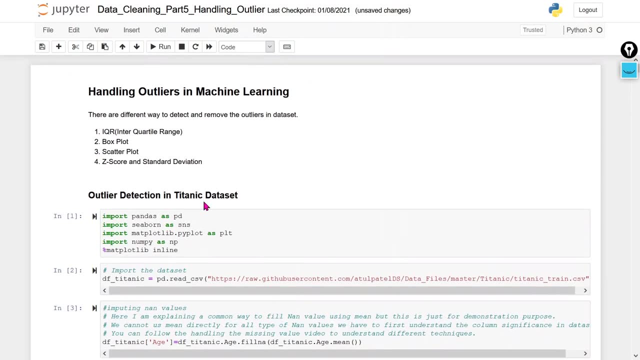 the outliers And by using the IQR and by using the standard deviation and z-score, we calculate the outliers. and once we calculate the outlier, we try to impute those outliers with the help of NAND value and once we have the null value, we can impute those null value as per our normal procedure. like most of the time, we try to remove. 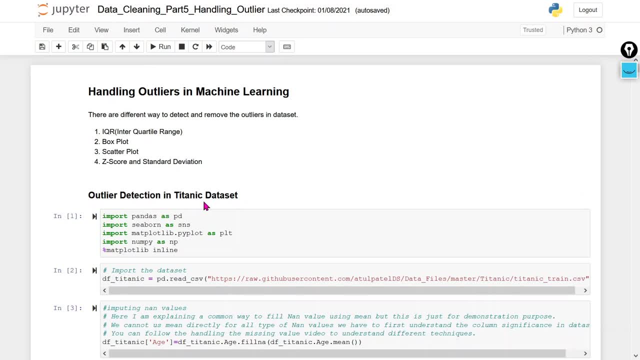 the outlier, but it is not a good approach to remove the outlier directly. it would always be recommended that before deleting the outliers or imputing the outlier that discuss with the domain expert. might be those outliers have some good information and those is required for your machine learning modeling. so just discuss with the domain expert before going to take any action on.